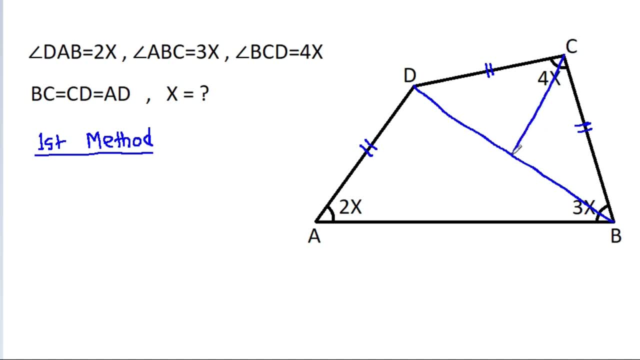 C on BD. Suppose this point is E, Then in any triangle ABC, if AB is equal to AC and if we draw a perpendicular AD on BC, then BD it will be equal to CD And also these two angles they will be equal. 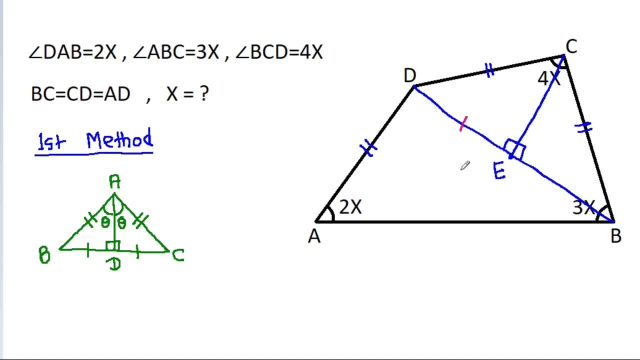 So here DE it will be equal to BE. suppose A and we have angle BCD is 4x. So these two angles they will be equal and 2x. And now if we draw a perpendicular from D on AB, suppose this point is F. Then if 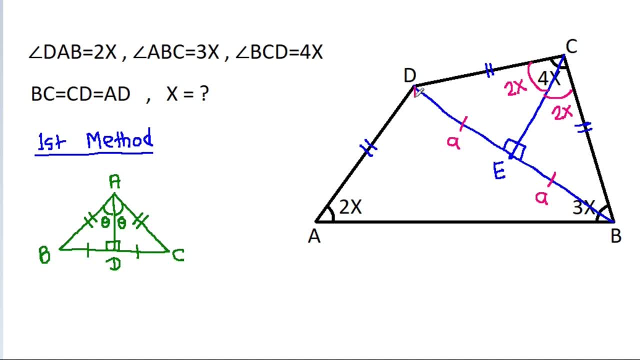 B is equal to AB and if we draw a perpendicular from D, we have angle BCD is 4x, And if we draw a perpendicular from AB, suppose this point is AB. Then if we draw a perpendicular from D on AB, suppose this point is F. 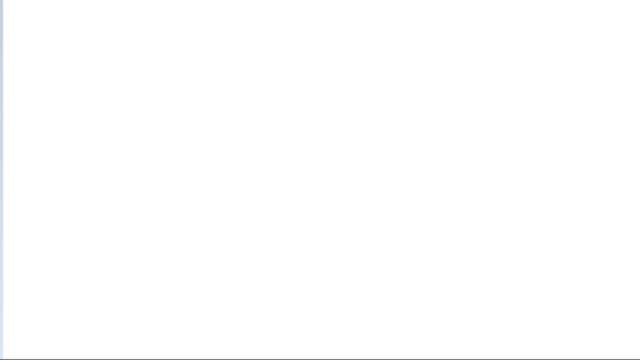 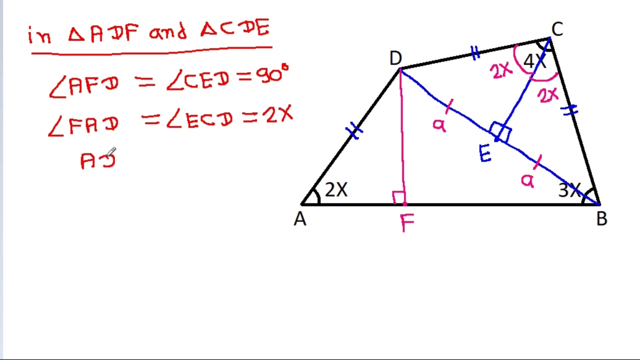 Now in triangle ADF and triangle CDE we have angle AFD is equal to angle CDE, That is 90 degree, and angle FAD, it is equal to angle ECD, that is 2x, and AD, it is equal to CD. 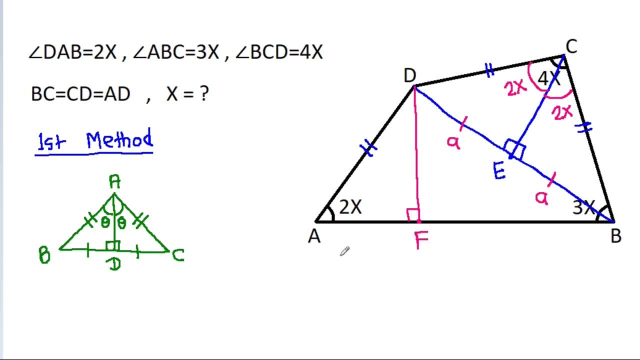 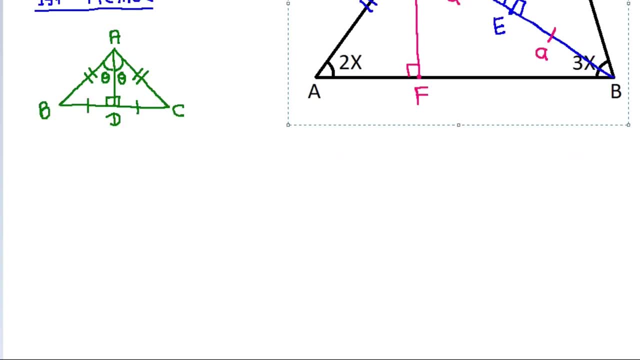 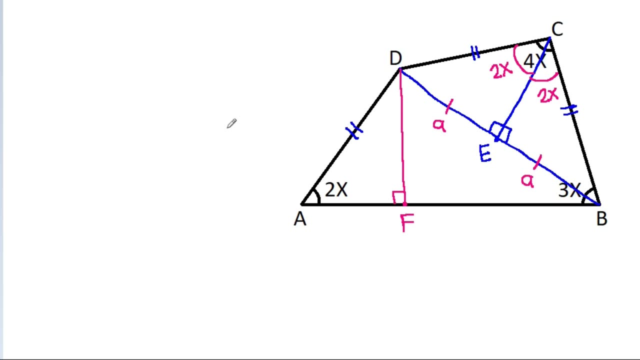 So here if I draw a perpendicular on AD and now if we draw a perpendicular from D on AB- Suppose this point is F- Then Now in triangle ADF and triangle CDE we have: angle AFD is equal to angle CDE. 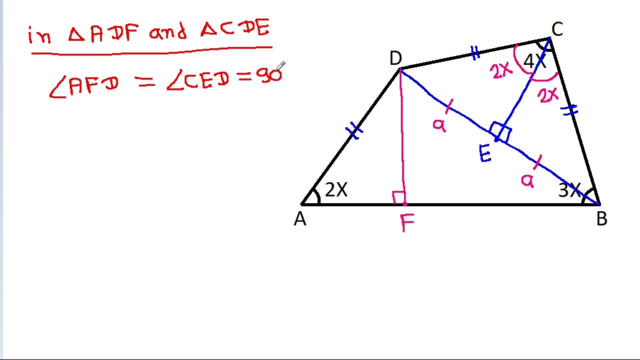 That is 90 degree, and angle FAD is equal angle ECD, that is two x, and AD is equal to CD. so there, angle ADF, it will be congruent to the angle CDE, That means DF, it will be equal to DE. 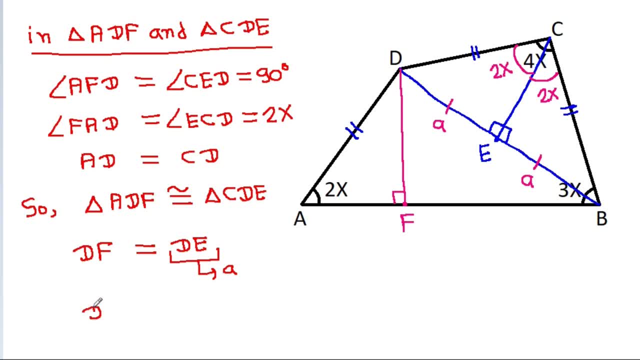 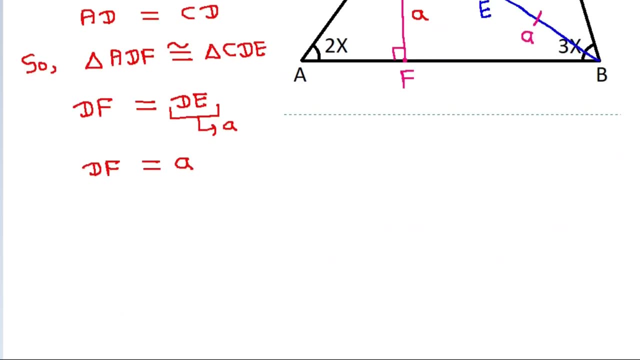 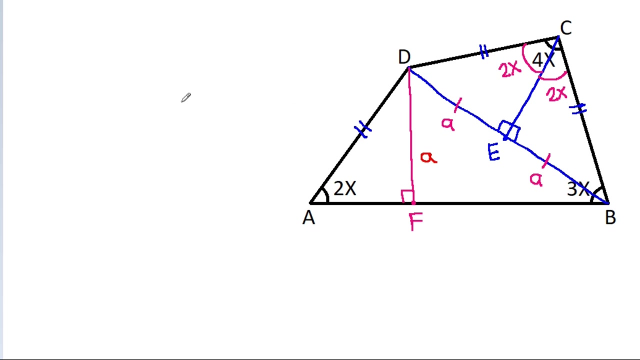 And DE it is A. So DF it will be equal to A, DF, it will be A. And now int angle: DE. Now int angle CDE, DFB, it is DFB. this angle is 90 degree. 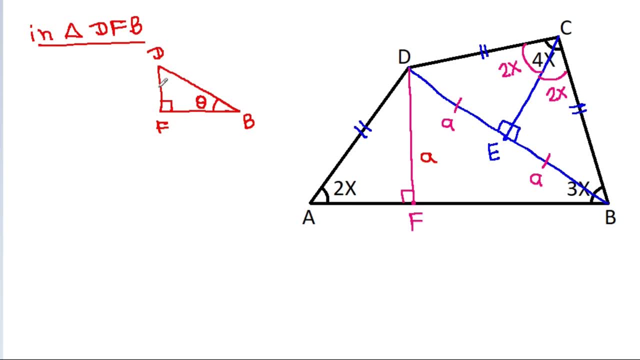 This angle, suppose theta and we have DF is A and DB, it is A plus A, that will be 2A. So sine theta it will be equal to DF by DB and sine theta it is equal to A by 2A. 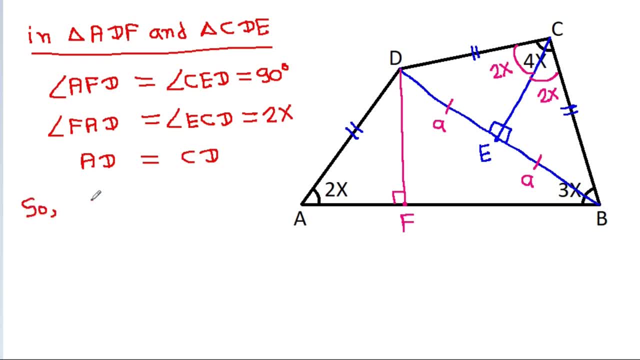 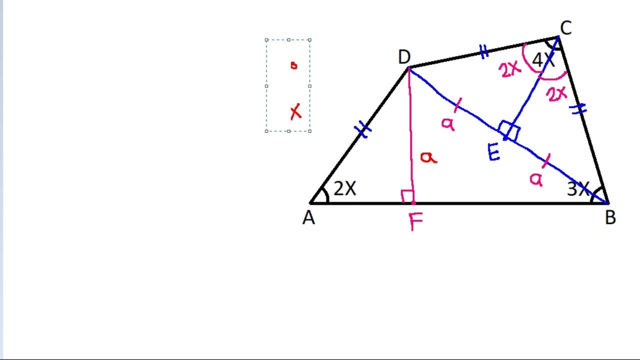 So triangle ADF, it will be congruent to triangle CDE. That means DF, it will be equal to DE, and DE it is A. so DF it will be equal to A, DF it will be A. And Now in triangle DFB, It is DFB. 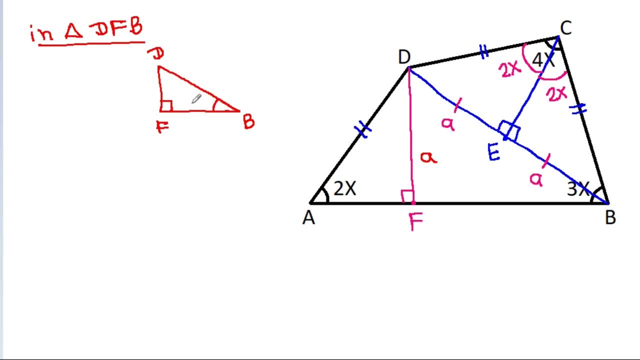 This angle is 90 degree. This angle, suppose theta and we have, DF is A And DB it is A plus A, that will be 2A. So sin theta it will be equal to DF by DB And sin theta it is 90 degree. 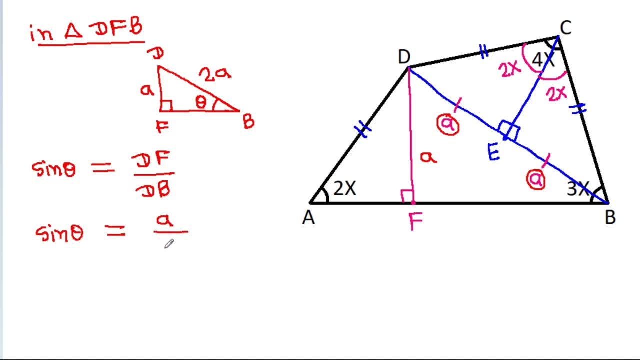 So sin theta it will be equal to DF by DB And sin theta it is 90 degree And sin 2A will be equal to 2A And sin 2A will be equal to deu. So this angle will be also 90 degree and 3x. 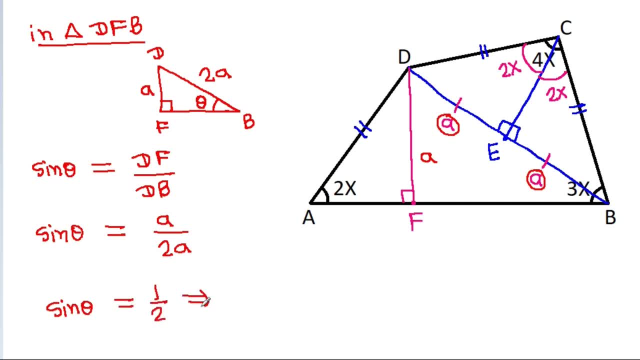 So we get sin: theta is equal to 1 by 2. That means theta it will be equal to 30 degree. So this angle: it is 30 degree. So this angle, it will be 3x minus 30 degrees. 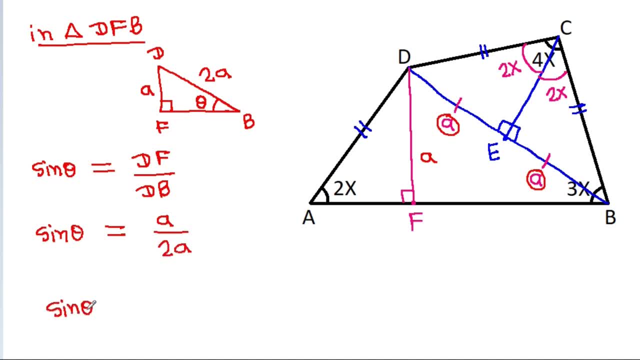 So we get sine: theta is equal to 1 by 2. That means theta it will be equal to 30 degree. Okay, Thank you, Bye, Thank you. So this angle, it is 30 degree. So this angle, it will be 3x minus 30 degree. 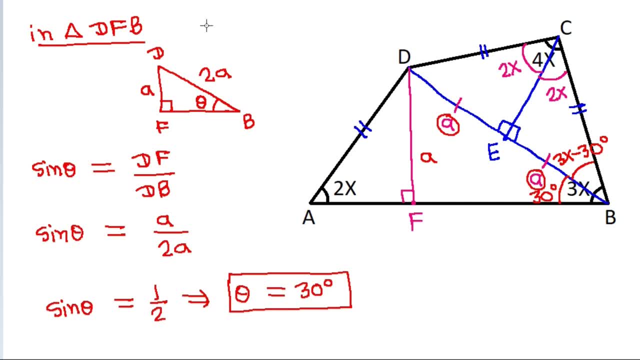 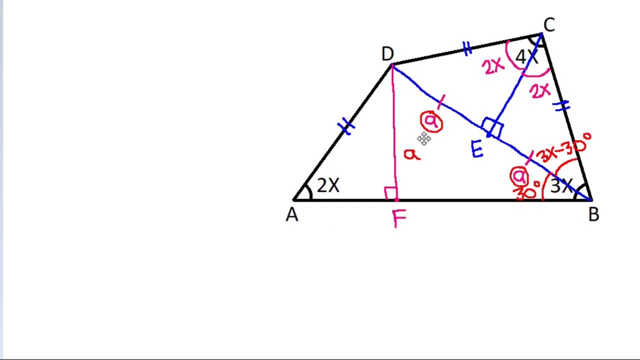 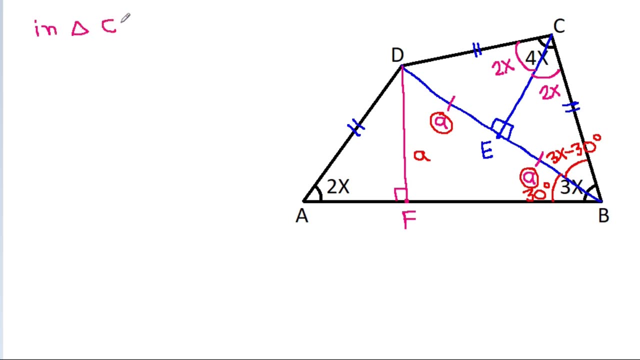 And now int angle: it will be 2A. Okay, So this is the angle. it is 30 degree. Okay, Bye, Bye, Bye Bye, CEB. It is CEB. This angle, it is 3x minus 30 degree. This angle is 2x and this angle. 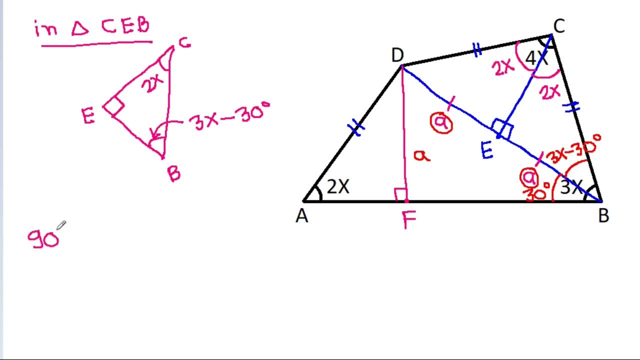 is 90 degree. So 90 degree plus 2x plus 3x minus 30 degree, it will be equal to 180 degree. And 90 degree minus 30 degree will be 60 degree plus 2x plus 3x will be 5x, That is equal to 180. 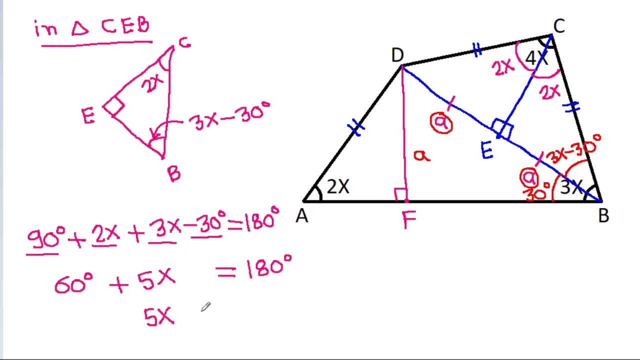 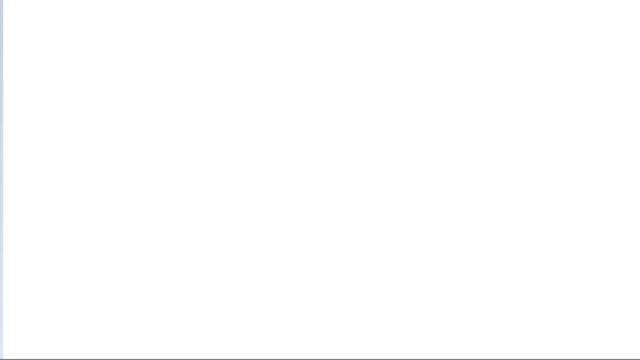 degree, So 5x, it will be equal to 120 degree, So x will be equal to 24 degree. And second method, we have B3.. A, B, C is equal to CD, is equal to AD, Suppose A. And now if we join BD, then in any triangle 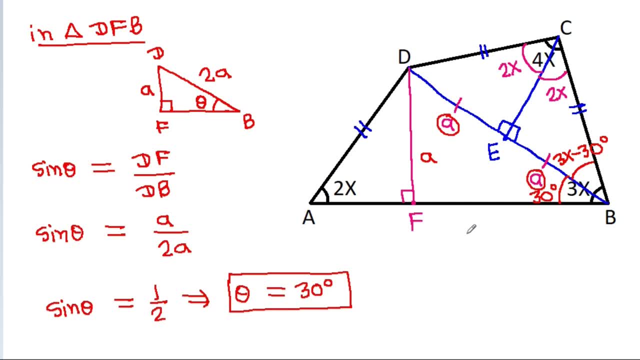 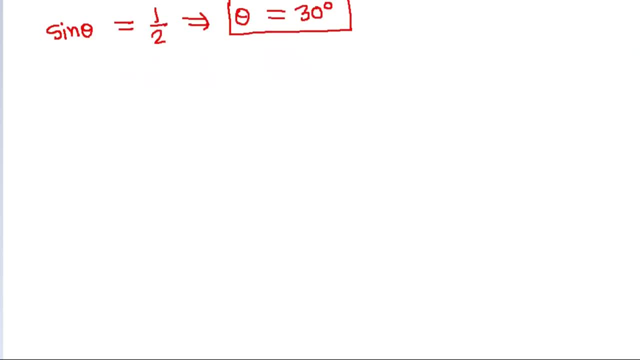 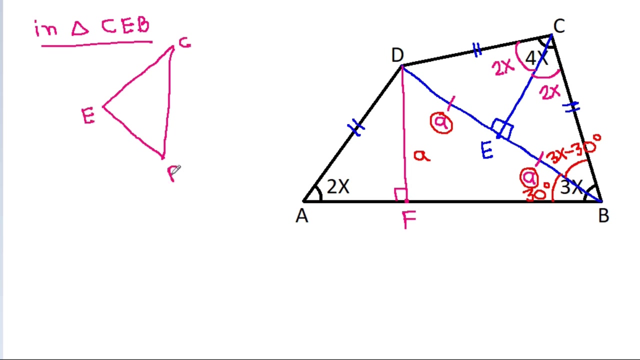 minus 30 degree. and now inter angle CEB. it is CEB, this angle, it is 3x minus 30 degree. This angle is 2x and this angle is 90 degree. So 90 degree plus 2x plus 3x minus 30 degree, it will be equal to 180 degree. 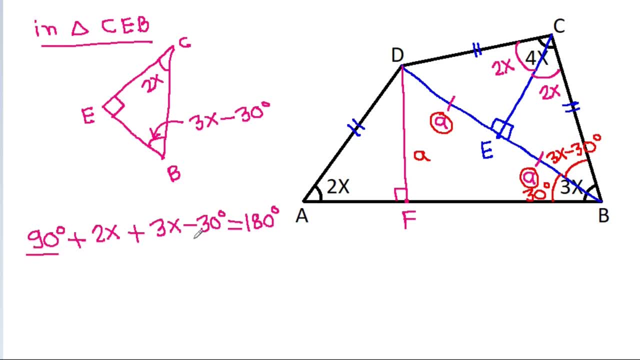 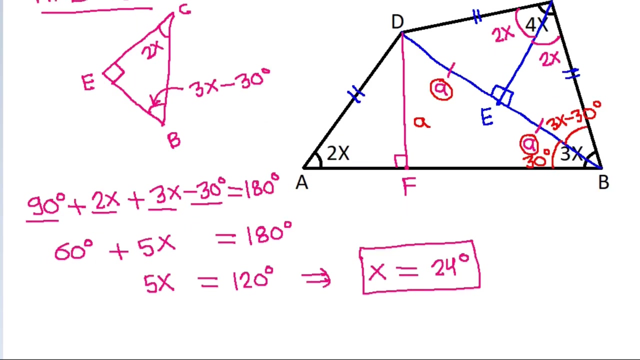 And 90 degree minus 30 degree will be 60 degree plus 2x plus 3x, 3x will be 5x. that is equal to 180 degree. So 5x, it will be equal to 120 degree. so x will be equal to 24 degree. 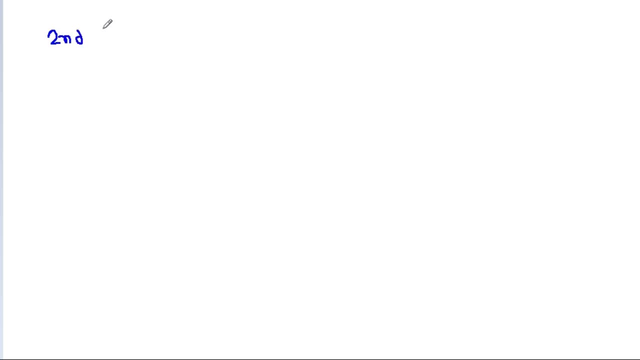 And second method. Okay, We have: BC is equal to CD is equal to AD, suppose A. and now if we join BD, then in any triangle, ABC, if AB is equal to AC, then these two angles they will be equal. 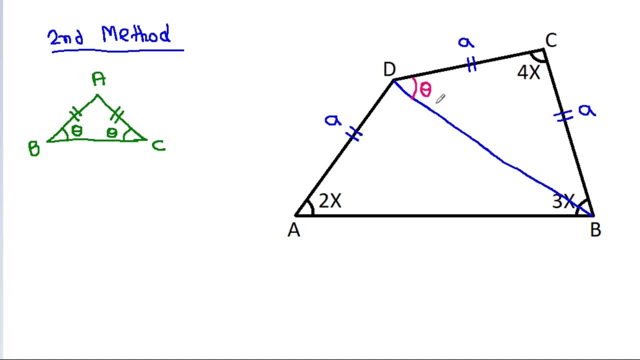 So here, if this angle is theta, then this angle it will be also theta. So this angle it will be 3x minus theta. And now, Okay, Okay, In any triangle, A, B, C, if BC is A, AC is B and AB is C, then A by sin, A it is. 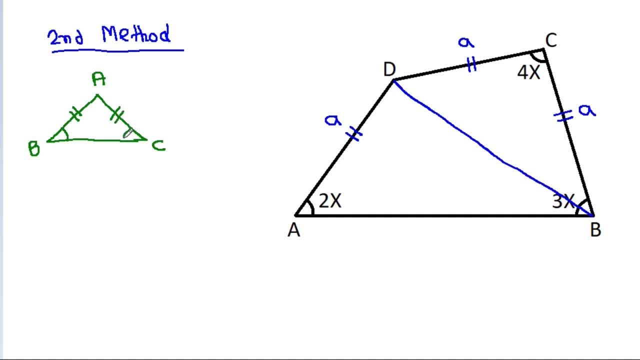 A, B, C. If A, B is equal to AC, then in any triangle, if A, B is equal to AC, then then these two angles, they will be equal. so here, if this angle is theta, then this angle it will be also theta, so this angle it will be 3x minus theta. 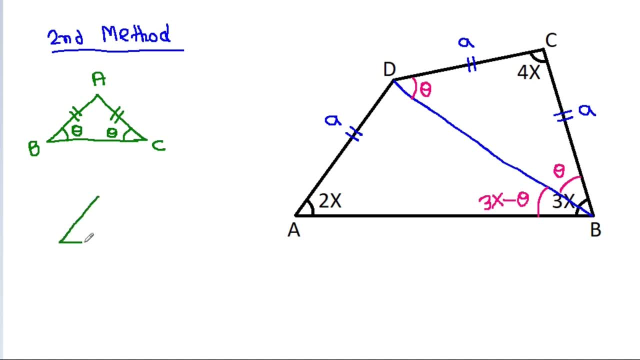 And now in any triangle, ABC, if BC is A, AC is B and AB is C, then A by sin A, it is equal to B by sin B, it is equal to C by sin B. Ok, Ok. 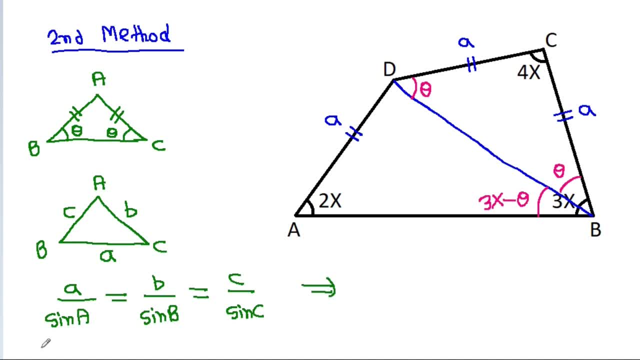 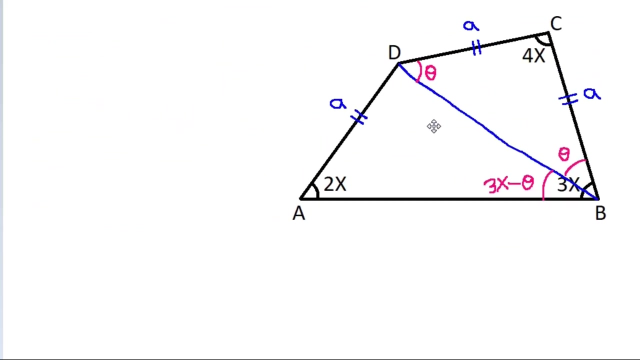 Ok, Ok, Ok. sin c, and from this equation we can get a by b, is equal to sin a by sin b, And here in triangle, ADB, AD by BD, it will be equal to sin 3x by sin b. 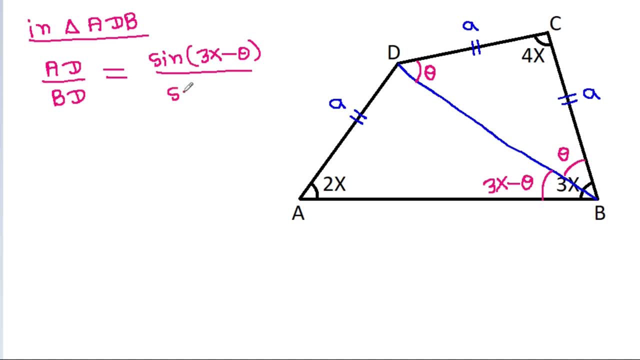 sin 3x minus theta by sin 2x and AD is a by BD it is equal to sin 3x minus theta by sin 2x. So BD it will be equal to a times sin 2x by sin 3x. 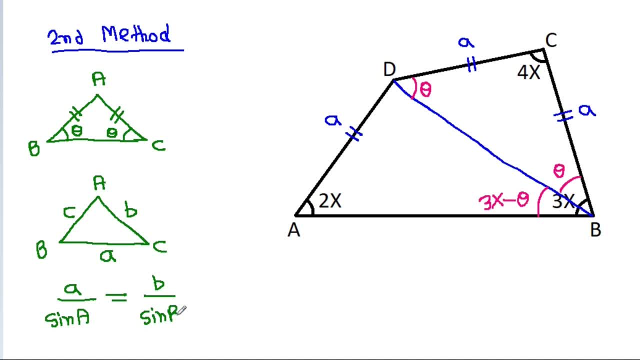 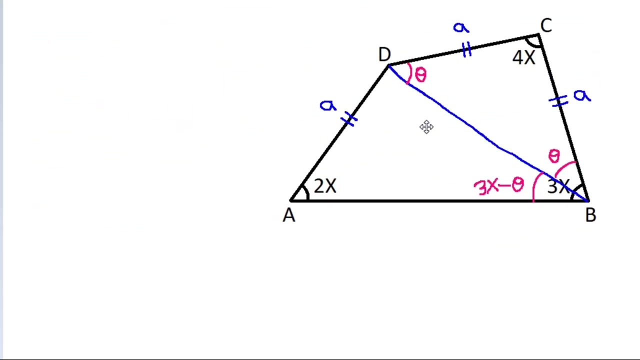 equal to B by sin B, it is equal to C by sin C. Okay, And from this equation we can get: A by B is equal to sin A by sin B, And here in triangle A, B, C, if BC is A, AC is B, then it is equal to B by sin B. 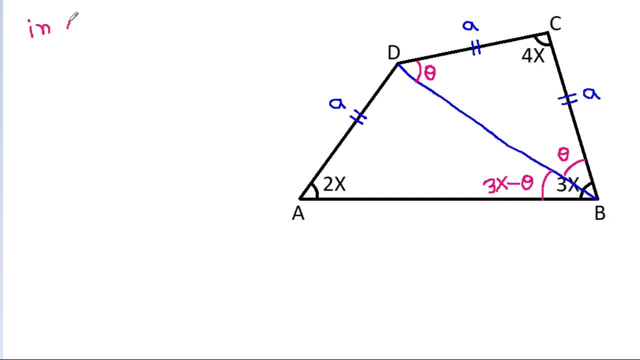 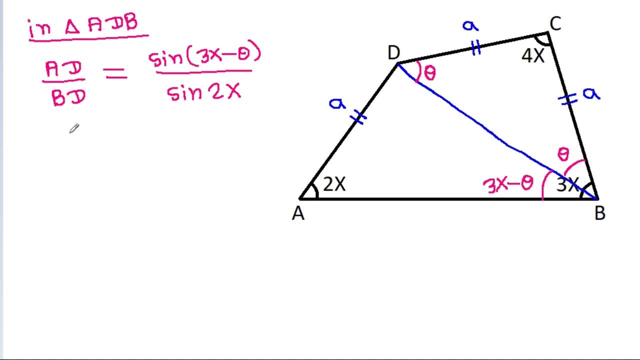 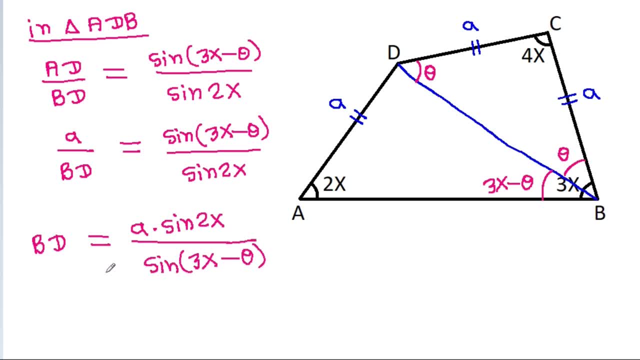 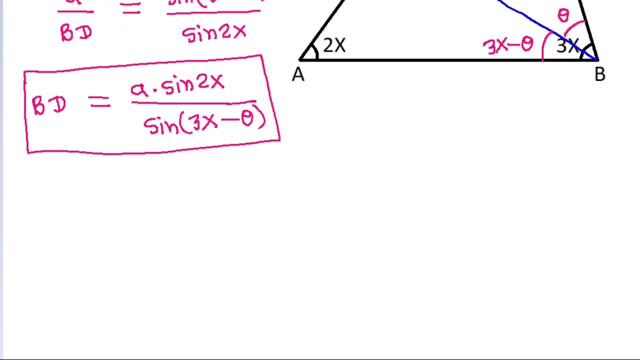 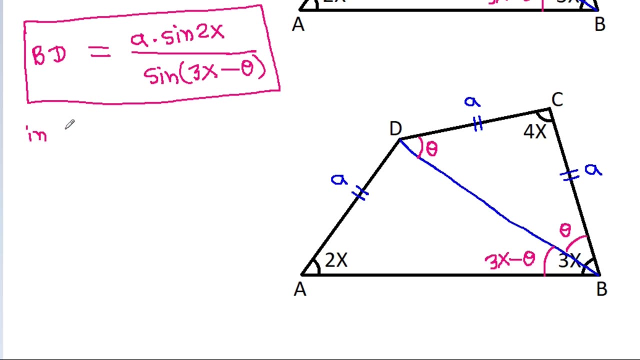 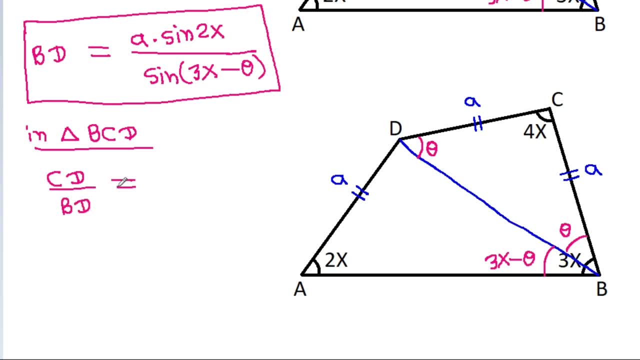 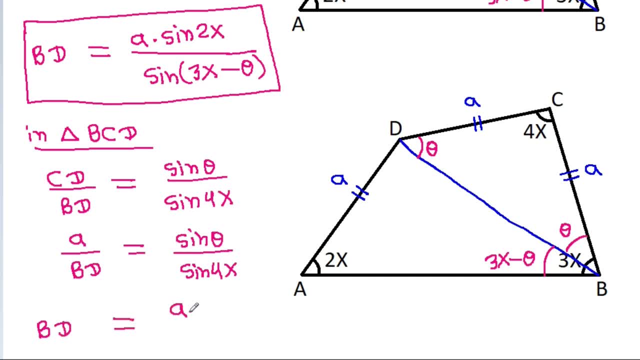 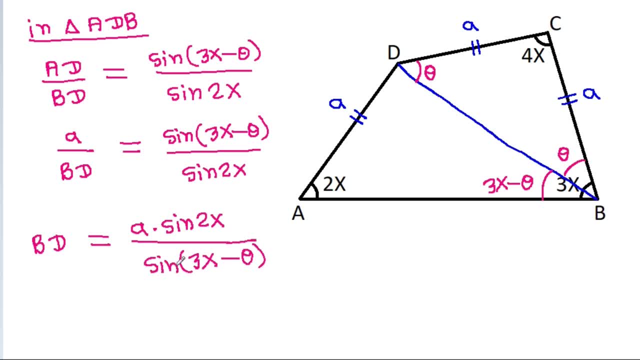 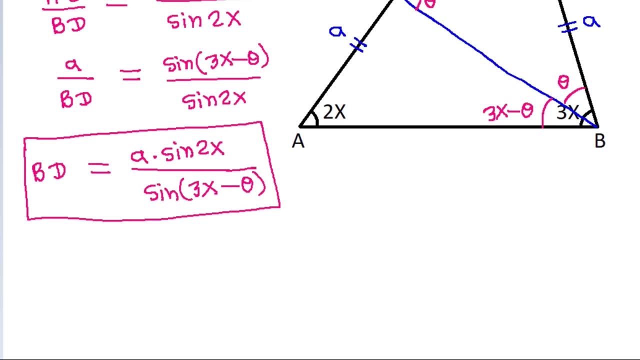 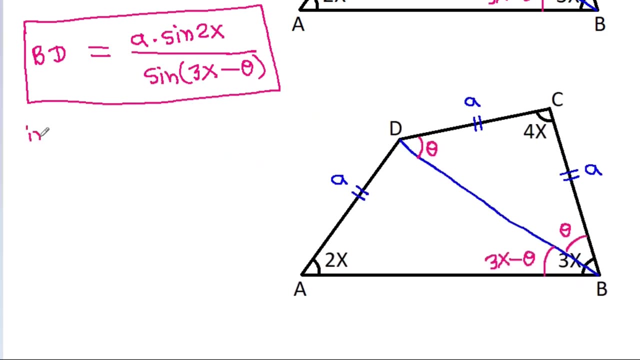 sin 3x minus theta. and now in triangle, BCD, CD by BD, it will be equal to sin 3x minus theta by sin 2x, It will be equal to sin theta by sin 4x. and CD is a by BD, it is equal to sin theta by sin 4x. 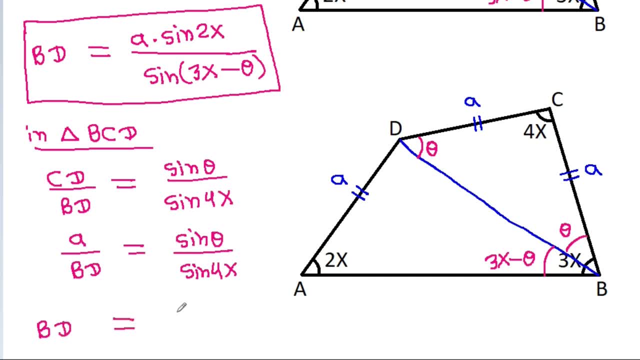 So BD it will be equal to a times sin 4x by sin 2x. And now suppose it is equation 1 and it is equation 2, then BD it will be equal to BD, So a times sin 2x by sin 3x minus theta. 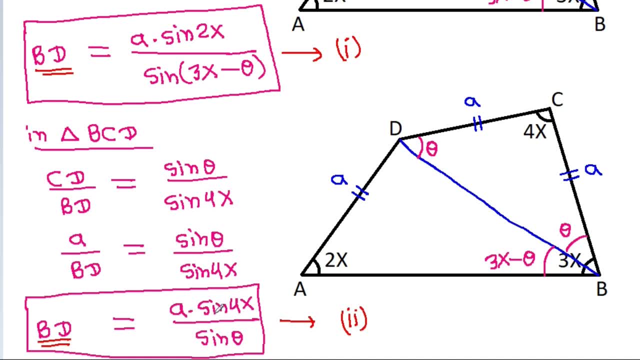 it will be equal to a times sin 4x by sin theta, Then BD. it will be equal to a times sin 4x by sin 3x minus theta, Then BD. it will be equal to a times sin 4x by sin 3x minus theta. 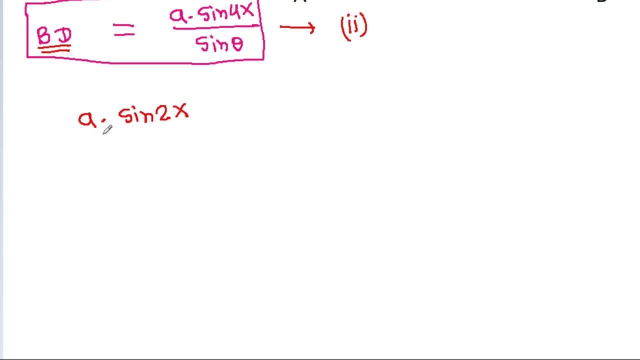 So a times sin 2x by sin 3x minus theta, it will be equal to a times sin 4x by sin theta. So a times sin 2x by sin 3x minus theta, it will be equal to a times sin 4x by sin theta. 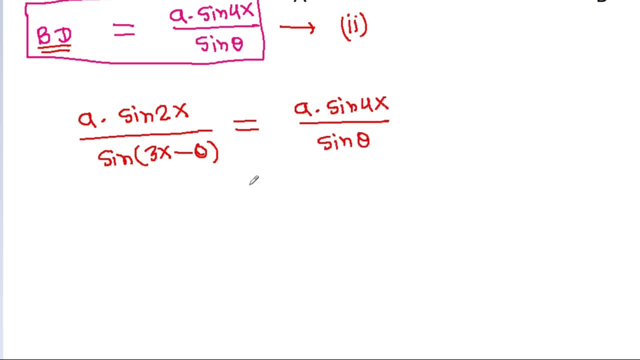 So a times sin 2x by sin 3x minus theta, it will be equal to a times sin 4x by sin theta. So a times sin 4x by sin 3x minus theta, it will be equal to a times sin 4x by sin theta. 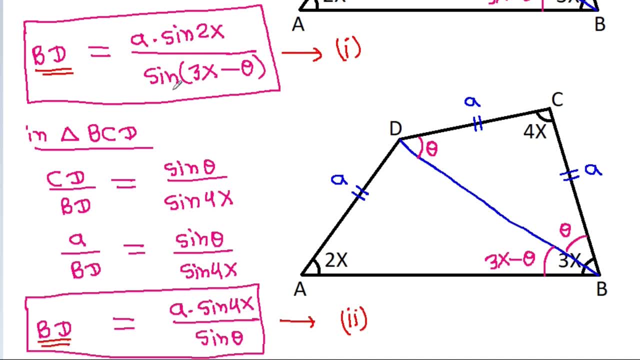 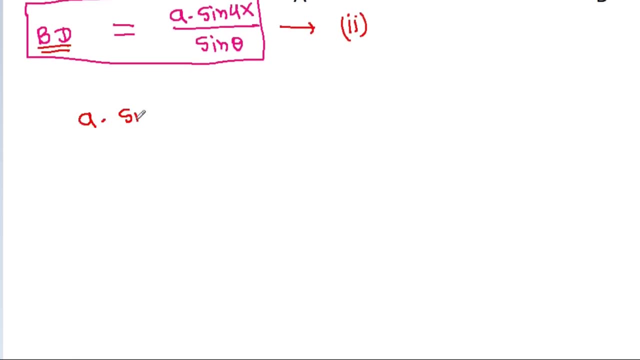 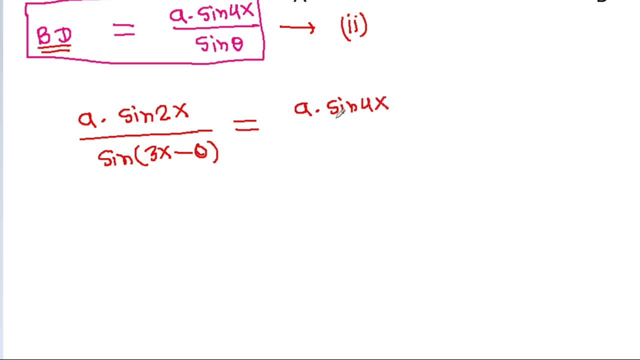 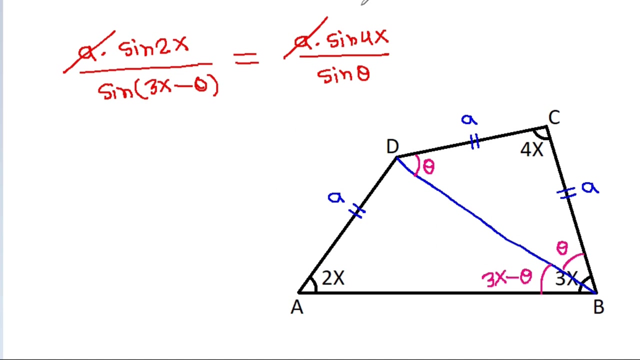 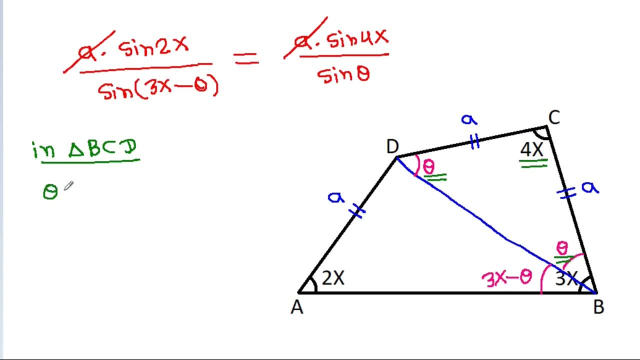 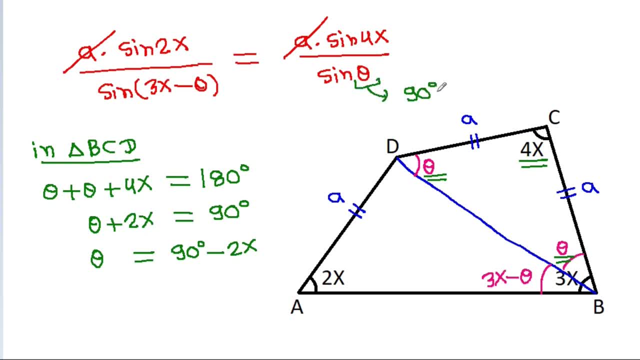 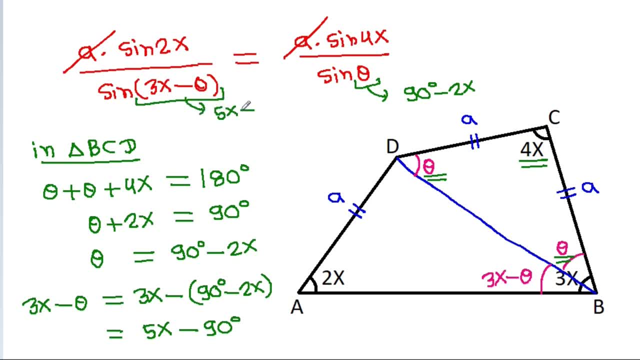 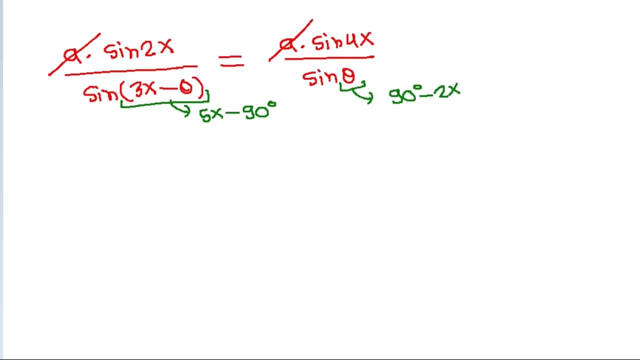 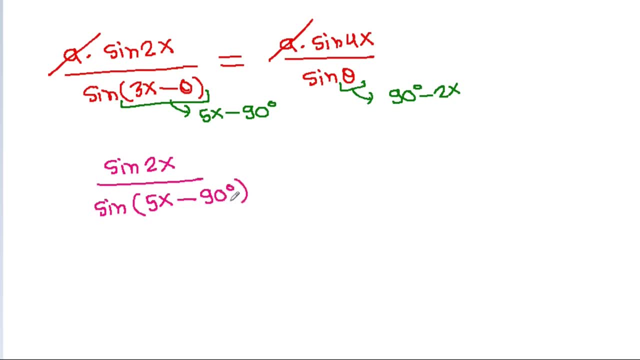 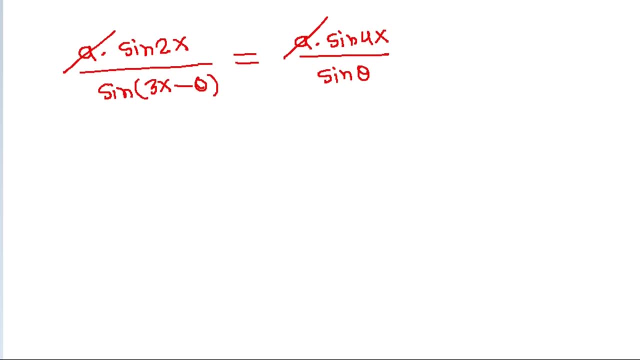 So a times sin 2x by sin 3x minus theta, it will be equal to a times sin 4x by sin theta. So a times sin 2x by sin 3x minus theta, it will be equal to a times sin 4x by sin theta. 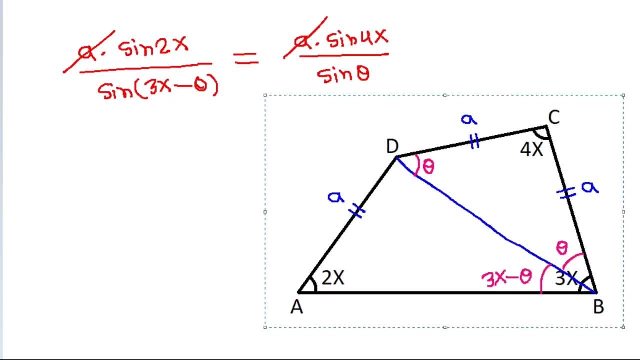 Here inter angle BCD: theta plus theta plus 4x. theta plus theta plus 4x, it will be equal to 180 degree. So theta plus 2x it will be equal to 90 degree. So theta, it will be equal. 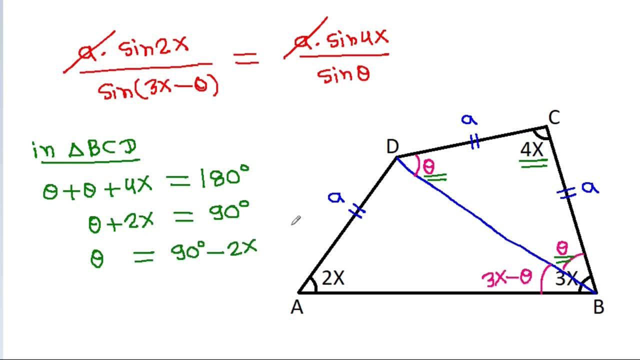 to 90 degree minus 2x Theta, it is 90 degree minus 2x, And 3x minus theta, it will be equal to 3x minus 90 degree minus 2x, That will be 5x minus 90 degree. 3x minus theta, it is 5x minus 90 degree. And. 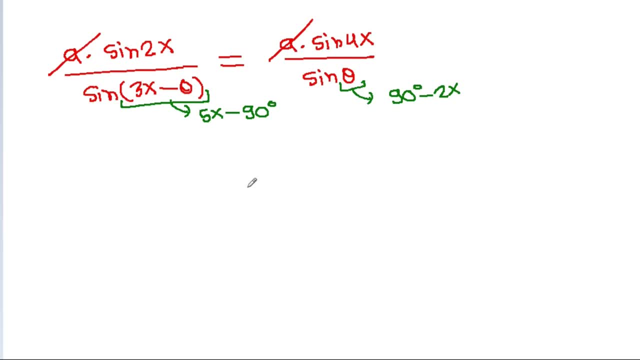 we have: sine 2x by sine 5x minus 90 degree is equal to sine 4x. by sine 90 degree minus 2x And sine of minus 4x. by sine 5x minus 90 degrees, it will be equal. 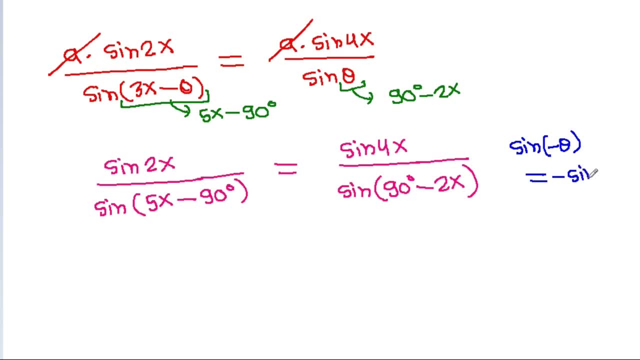 2x minus 3x. responders, be careful when you make this process because the strokes should be 6x and 900 degree over a remote. So if the gemeins도 are 5x, it will be equal theta. it is equal to minus sin theta, So it will be sin 2x by minus sin, 90 degree minus. 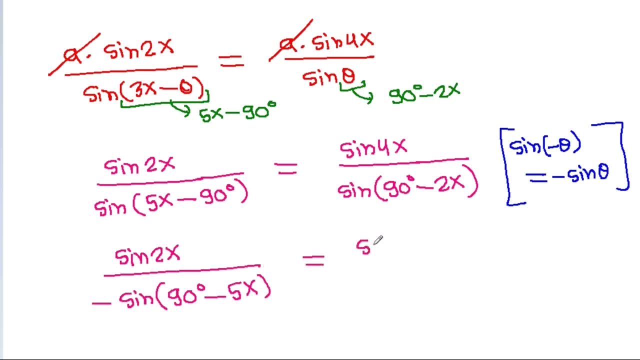 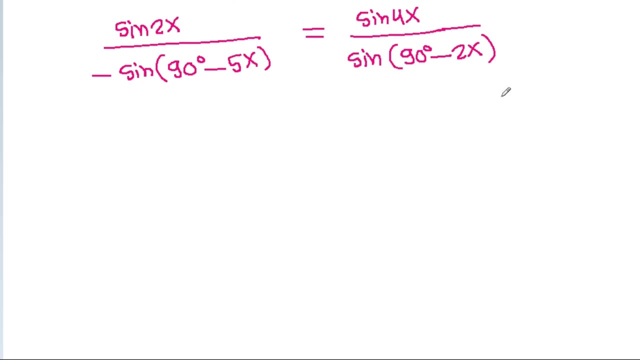 5x is equal to sin 4x. by sin 90 degree minus 2x And sin 90 degree minus theta, it is equal to cos theta. So it is sin 2x by minus cos 5x is equal to, and sin 4x it will be 2 times sin 2x times. 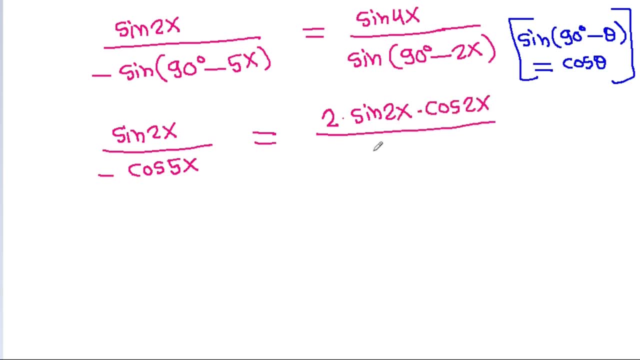 cos 2x by this will be cos 2x, Because sin 2a it is equal to 2x sine a cos a, and now cos 2x will get cancelled. Sine 2x will get cancelled, So we get minus 1. 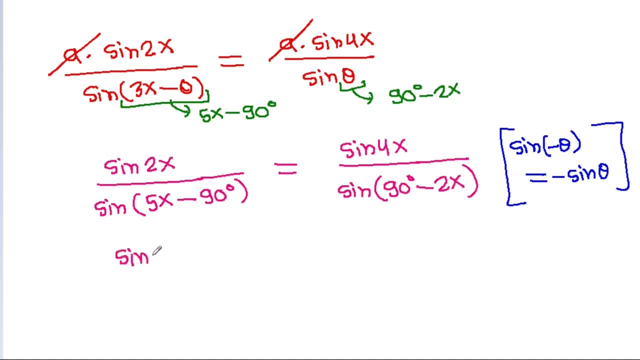 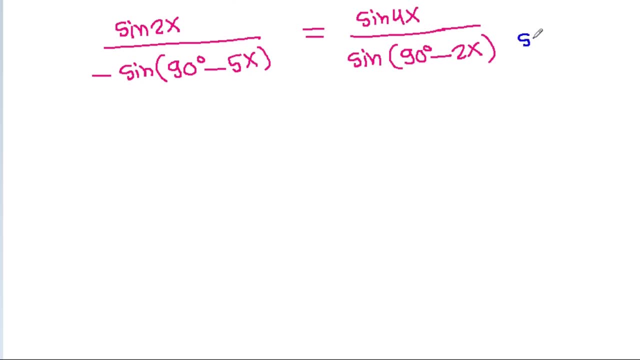 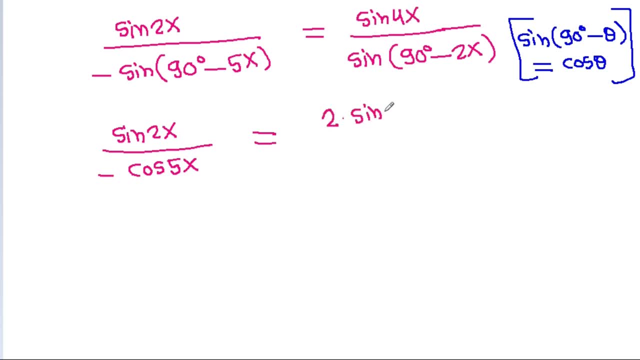 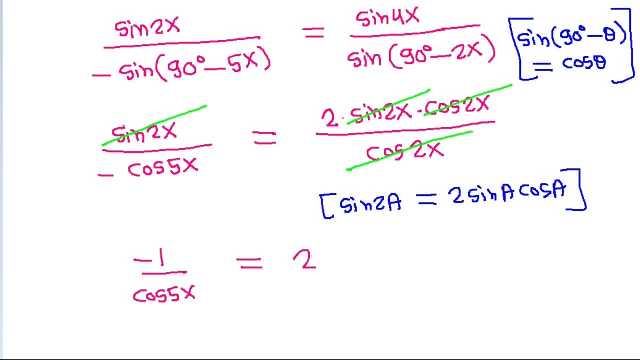 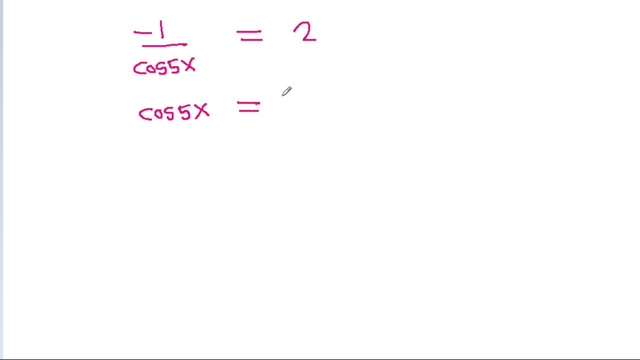 equal to 2, so cos 5x it will be equal to minus 1 by 2, and cos 60 degree it is 1 by 2, cos 120 degree it is minus 1 by 2 and cos 240 degree it is. 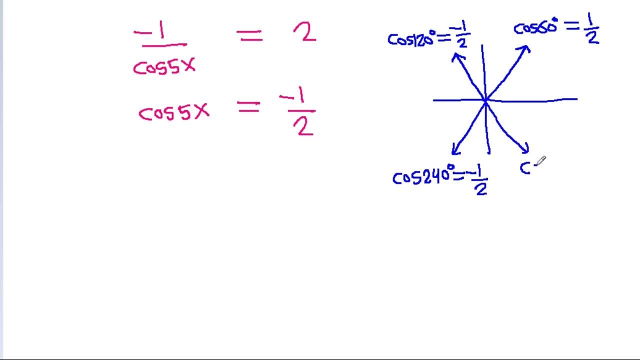 minus 1 by 2 and cos 300 degree it is 1 by 2 and we have cos 5x is minus 1 by 2, so 5x it will be equal to 1 divided by 2, 120 degree, 240 degree, and it can be 2n pi plus 120 degree and 2n pi plus 240 degree.